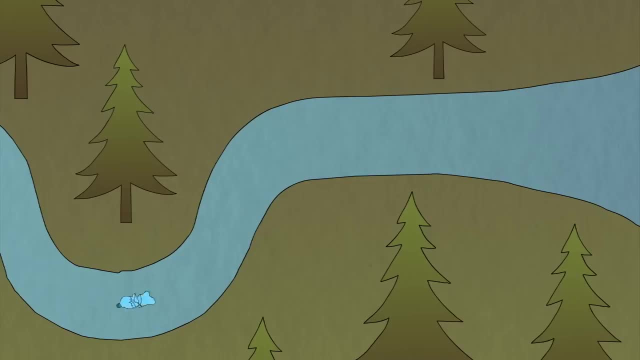 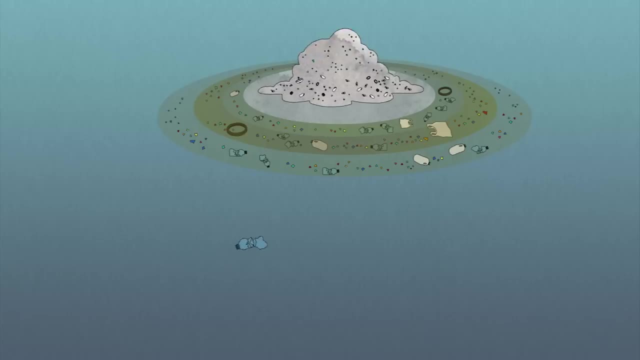 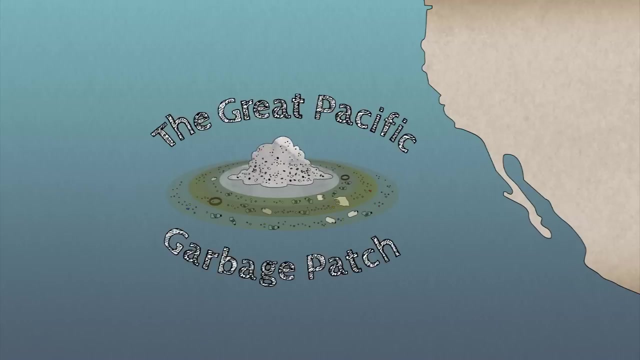 a trickle that reaches a stream, a stream that flows into a river and a river that reaches the ocean. After months lost at sea, he's slowly drawn into a massive vortex where trash accumulates, a place known as the Great Pacific Garbage Patch. 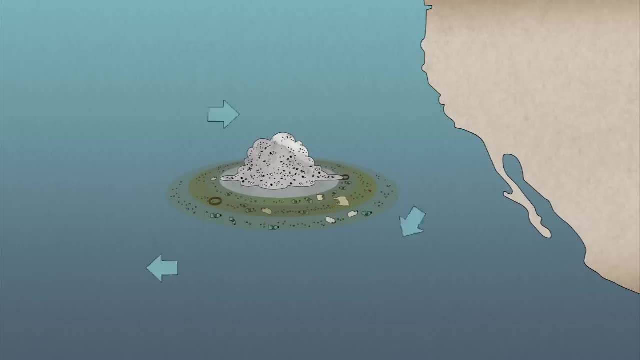 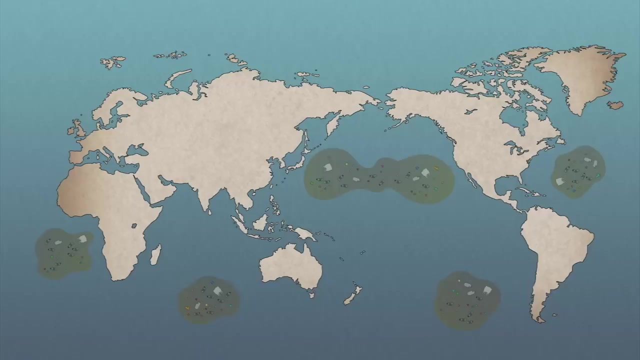 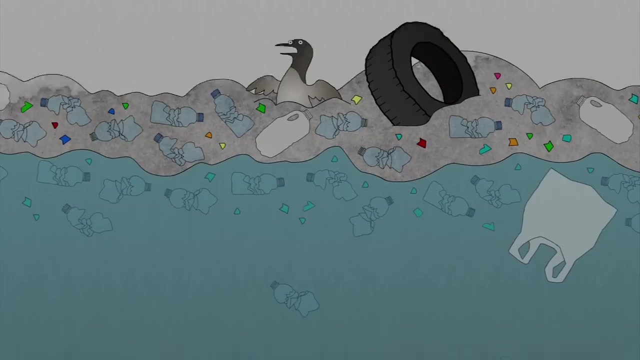 Here the ocean's currents have trapped millions of pieces of plastic debris. This is one of five plastic-filled gyres in the world's seas, places where the pollutants turn the water into a cloudy plastic soup. Some animals, like seabirds, get entangled in the mess. 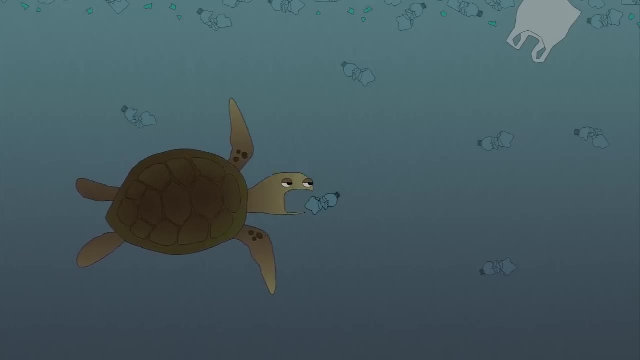 They and others mistake the brightly colored plastic bits for food. Plastic makes them feel full when they're not, so they starve to death and pass the toxins from the plastic up the food chain. For example, it's eaten by lanternfish. 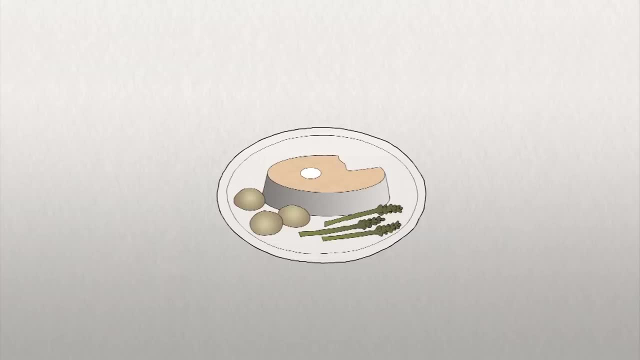 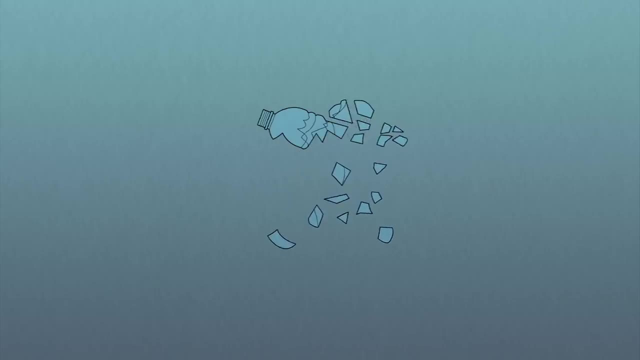 the lanternfish are eaten by squid, the squid are eaten by tuna and the tuna are eaten by us. And most plastics don't biodegrade, which means they're destined to break down into smaller and smaller pieces, called microplastics, which might rotate in the sea eternally. 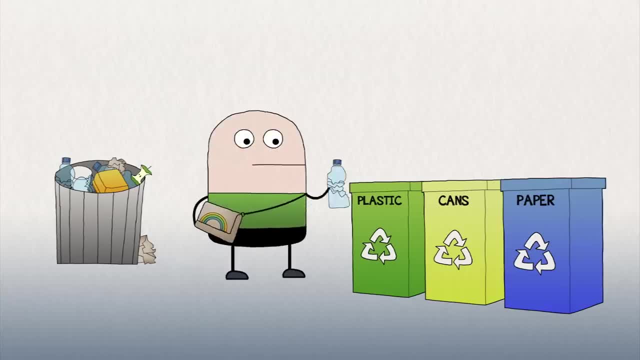 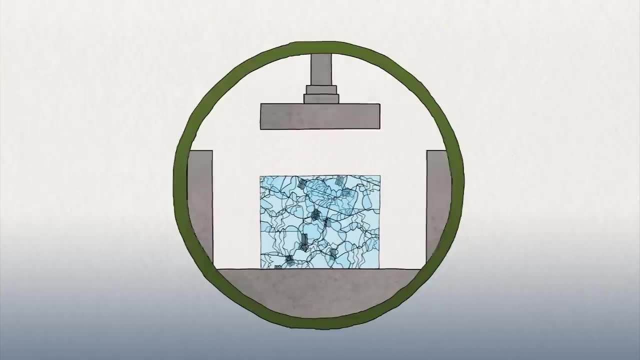 But Bottle 3 is spared the cruel purgatories of his brothers. A truck brings him to a plant where he and his companions are squeezed flat and compressed into a block. Okay, this sounds pretty bad too, but hang in there, it gets better. 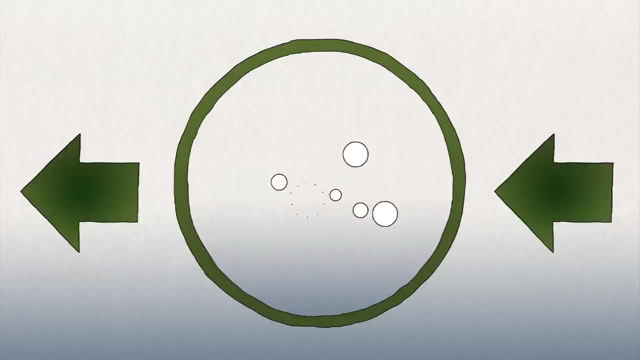 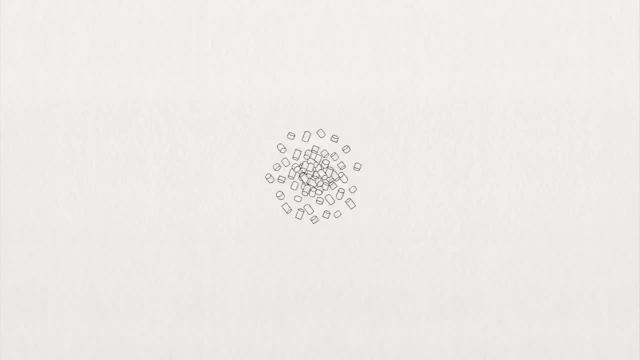 The blocks are shredded into tiny pieces, which are washed and melted so they become the raw materials that can be used again. As if by magic, Bottle 3 is now ready to be reborn, as something completely new For this bit of plastic with such humble origins. 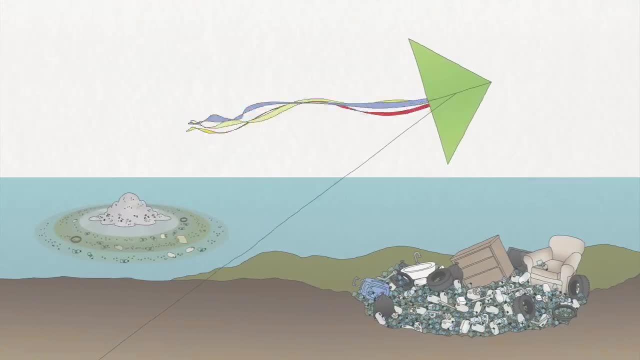 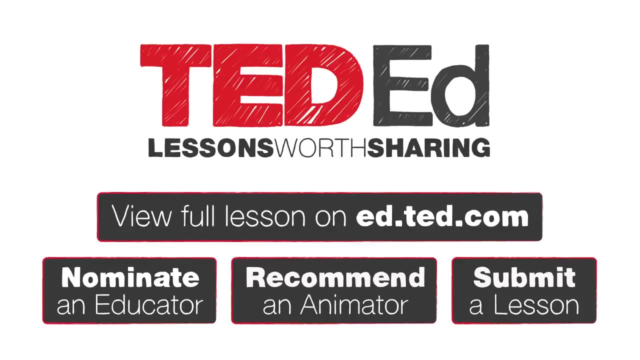 suddenly the sky is the limit. Subtitles by Subtitle Workshop.